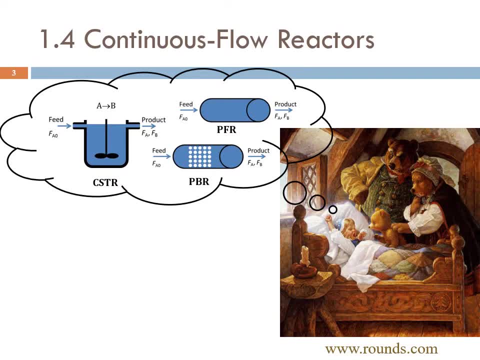 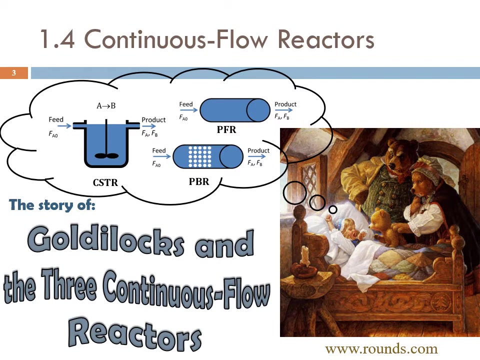 and a packed bid reactor, PBR. And then you know she tries the first reactor and it's too small, And then tries the last one. It's just right. right, It's just perfect. That's the story of Goldilocks and the three continuous flow reactors. So let's see what is the story about. 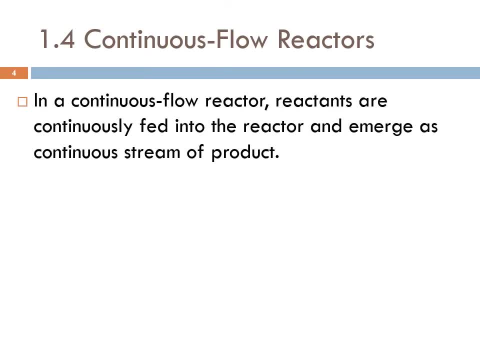 Well, in a continuous flow reactor, reactants are continuously fed into the reactor and emerge as continuous stream of product, So continuously they have input and continuously have output. Continuous flow reactors are almost always operated at a steady state. Of course, you know that the best thing about continuous devices, or 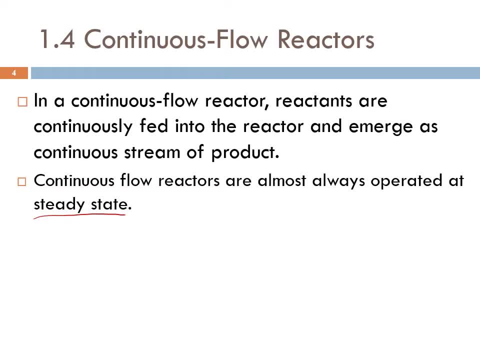 continuous equipments or the equipments that run continuously, the best thing for operation is to operate them under steady state, because then nothing is changing with time. You don't have to go through transient dynamic operation. right, You need everything to be steady, You need the process. 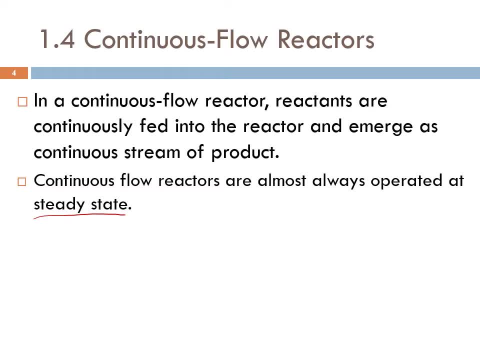 variables to be constant at the design values. You don't want change to happen. So continuous flow reactors: the same thing. You want to operate it at steady state. However, during the startup and shutdown it goes through a steady state operation. We will consider three types in the continuous flow. 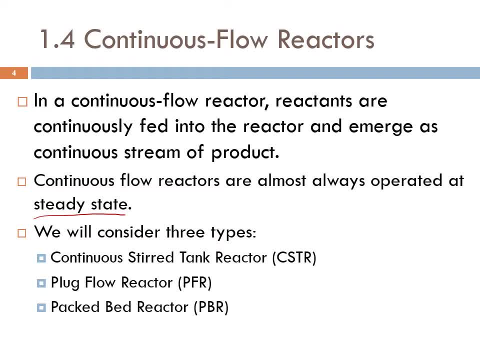 reactors. as I mentioned, It's that continuous stirred tank reactors, CSTR, plug flow reactor PFR and packed bed reactor PBR. Okay, the last two Shabab can be referred to as two-blur reactors, which you get to know now in. 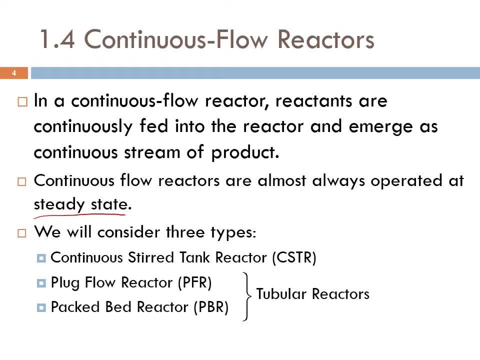 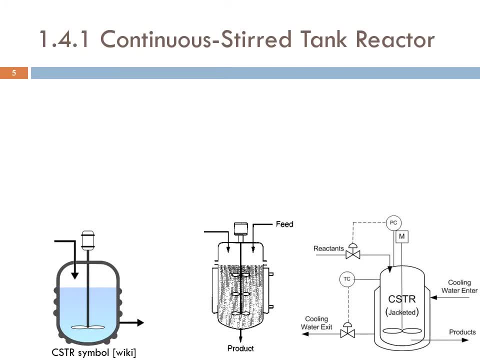 the following lecture why it is called so Okay, continuous stirred tank reactors. As you can see, it can be symbolized in one. any of these guys symbols schematic diagrams For those who are taking control. they can relate why we have all of that stuff. 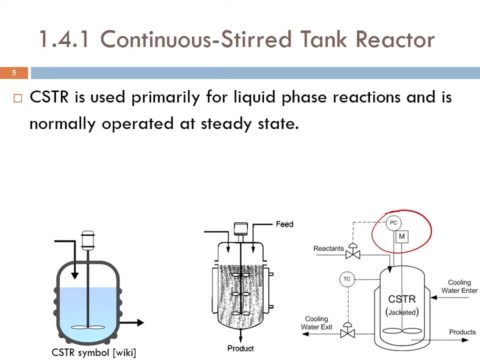 CSTR is used primarily for liquid phase reactions and is normally operated at steady state. It is assumed to be perfectly mixed. Again, we have an agitator and it's continuously mixing. we end up with perfect mixing. so what does that mean? yeah, you're right that. 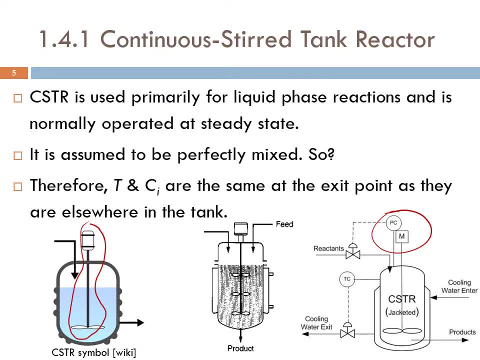 means that the temperature and the concentration inside the reaction inside the reactor here is the same everywhere. so it's not time of not function of volume, right? so temperature and concentration are the same everywhere and therefore the rate of reaction is same everywhere. so you have a uniform rate of reaction. so it's it's spatially constant, okay, and variable. 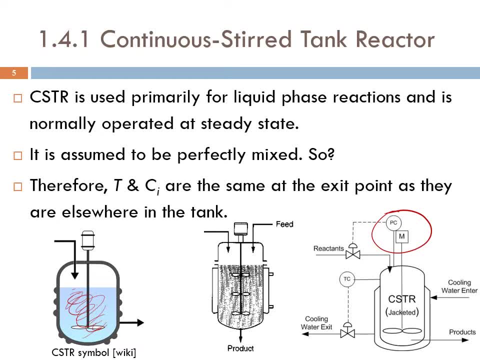 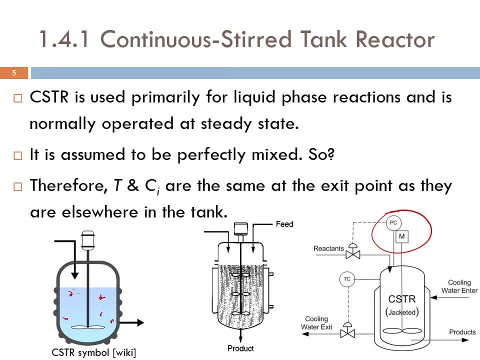 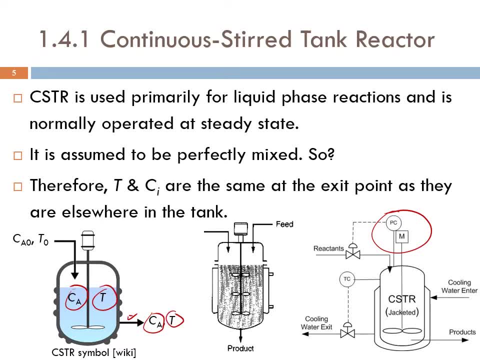 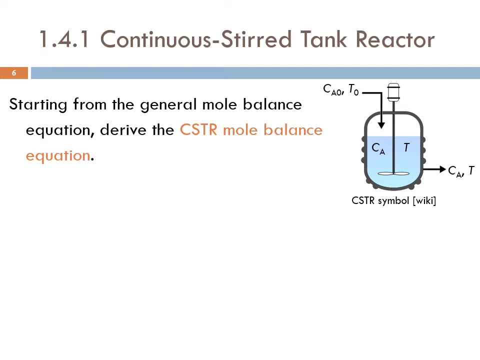 stream. the same thing is true for the temperature, okay, but of course they are different than the entering concentration and entering temperature. so therefore, temperature and concentration are the same at the exit point as they are elsewhere in the tank. okay, starting from the general model balance equation, drive the CSTR Moll. 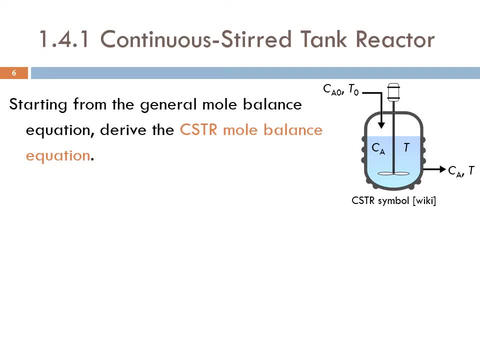 balance equation. let's do this together. so the general Moll balance equation- input F A0 minus output, F A plus generation, which is integration of R A dv from 0 to V, equals accumulation, which is d in A by dt. okay, let's look at some other. 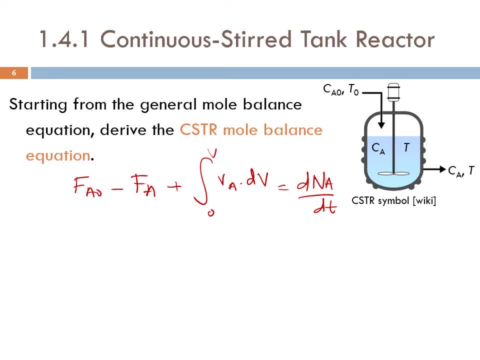 equations, the accumulation term, dna by dt. i say accumulation of what? that's the accumulation, accumulation of number of moles, of a correct number of moles of a where inside the reactor, inside my system, because i'm doing balance around the system, around the reactor, right, so that's input to the reactor. 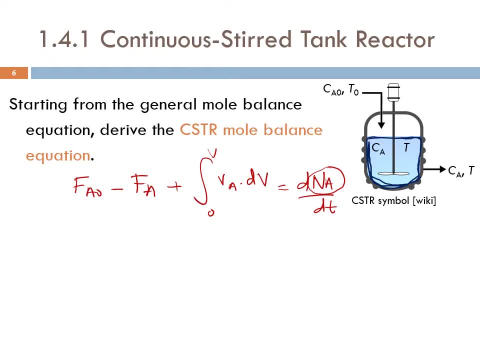 minus output from the reactor. that's the input, that's the output plus generation duration. where within the reactor, right equals accumulation where within the reactor. so that's number of moles of a inside the reactor. and is it zero? obviously not. we have some in a, we have a reaction. 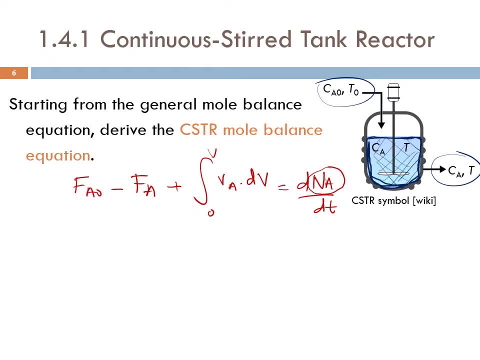 right. okay, so we have some a reactant to minimum and, and it's not zero. however, however, the change, the change of n? a with time, is zero. the change of n a with time is zero. why is that? because it's operated under steady state right. what does steady state operation means? steady state operation means the process variables do. 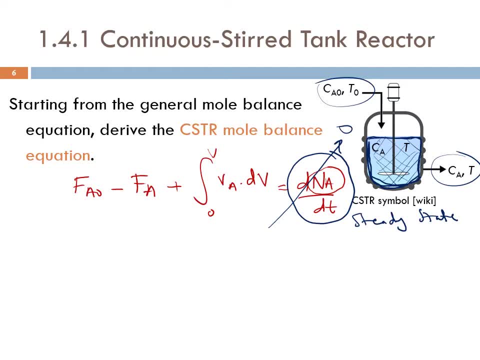 not change with time process variables like what, like ca, like na, like t, okay, so they are not changing with time. so therefore, in this case, dna by dt equals to zero. okay, can i simplify more? yes, we can. let's try f a, not minus f a. and what about r a? is r a? 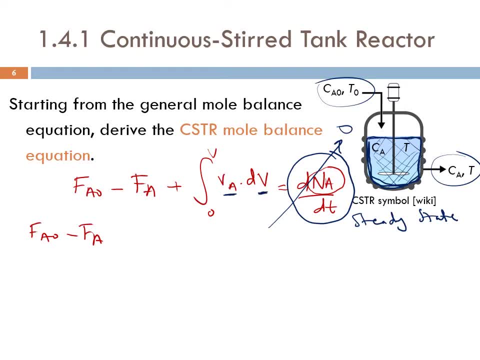 function of volume. we know that it's not correct because r is the same everywhere and this time an additional two values: f and r are the same everywhere and this time an additional two to RA being uniform throughout the reactor. It's also not changing with time because the system is operated under steady state. 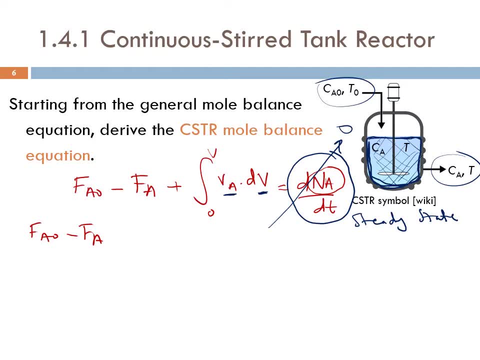 Okay, so RA goes outside the integration and we do the integration. we end up with: RA times V equals to zero. Let's take this term to the other side and we write it as: FA0 minus FA equals minus RA times V. What am I interested in when it comes to design of a reactor? 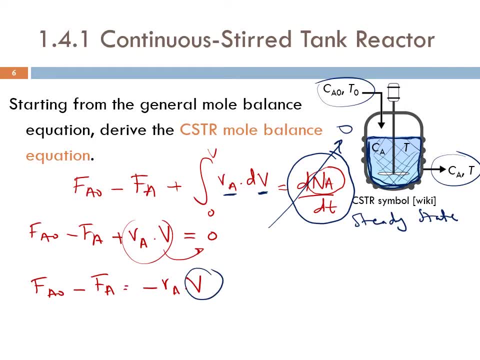 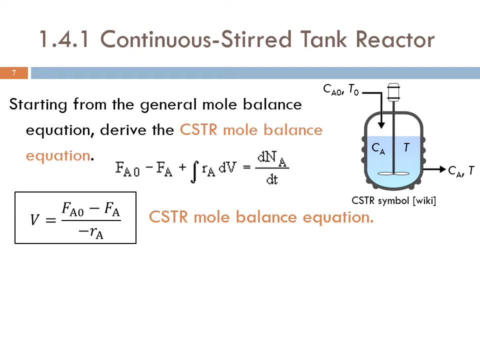 I'm interested in calculating the volume of the reactor. Therefore I write the equation as: V equals FA0 minus FA divided by RA. Okay, so now we have a design equation. There we go: CSTR mold bass equation or CSTR design equation. CSTR design equation. 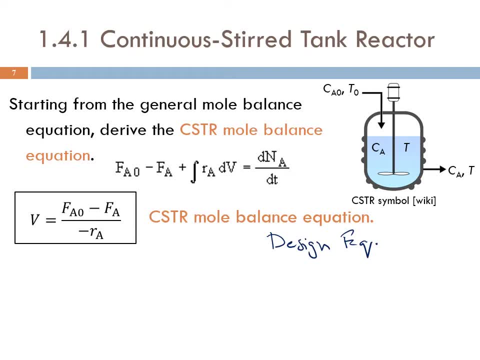 Okay, what's the story of this equation? So, in this course, about every component, Every question has a name, Every question has a story to tell. Okay, let alone that you will develop feelings toward these equations and you'll know, you'll. 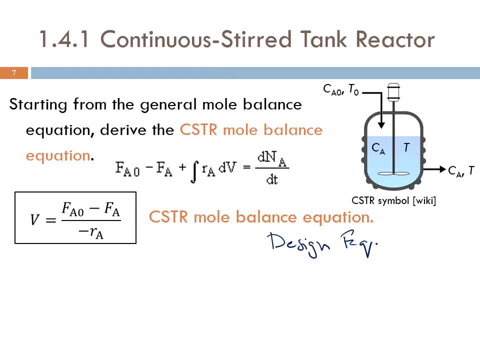 feel what will happen if this happened, What will you know, what's the response for this change, and so on. Okay, so what's the story of this equation? Well, simply here, the equation, the design equation. Okay, 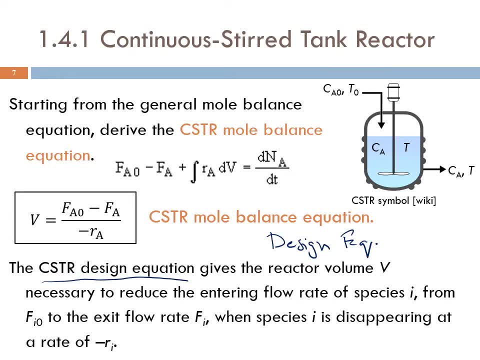 The CSTR design equation. the CSTR design equation gives the reactor volume necessary to reduce the entering molar flow rate of a species I or A in this case, from an initial value to that exit value. right, This is FA here. 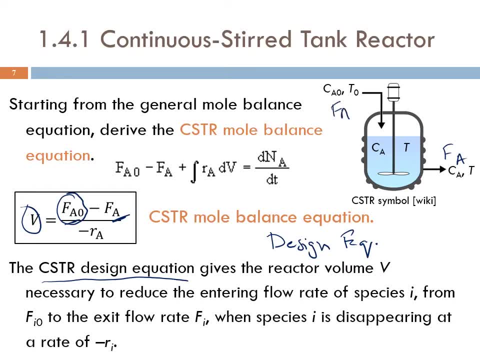 This is FA. Where is FA0?? FA0 is here. Okay, so it reduces it from A. Okay So it reduces it from A. Okay So it reduces it from A. Okay So it reduces it from FA0 to FA. reduces the molar flow rate from FA0 to FA at the exit. 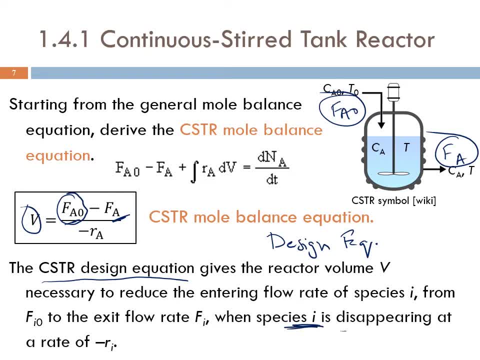 When a species I is disappearing disappearing see minus RA or minus RI. disappearing When a species I is disappearing at a rate of minus RI or minus RA if we're talking about A. So that's the story of this equation, Okay. 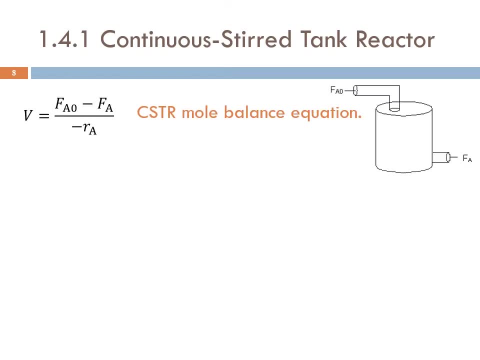 So that's the story of this equation. Great, So let's have some insight into this equation, the design equation for CSTR. Okay, let's solve for FA. When we solve for FA, we get this equation: FA equals FA0 plus V times RA. 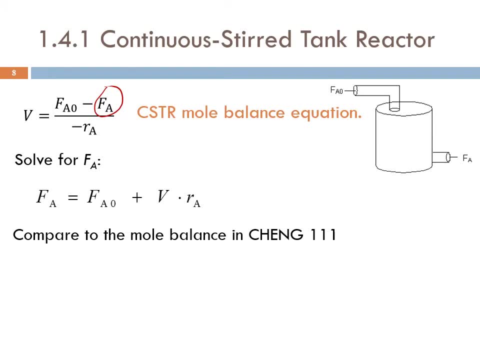 And let's compare this equation, Okay, to the mole balance equation that we have derived in introduction to chemical engineering, the first course on chemical engineering, remember, we got this equation. so let's see the similarity between these equations. here we have output f a equals input, which is f a naught. 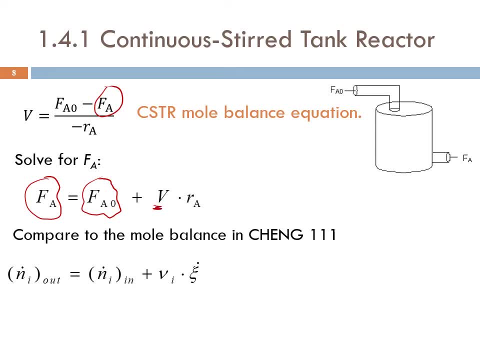 plus v, which is the volume, times r, a, which is the rate of reaction. okay, let's compare it to the equation we derived in triple one, and it's again the output: f and i dot. output equals input, right, but this time plus nu i, which is the stoichiometric number, stoichiometric number times zeta, times zeta dot. of course again, because 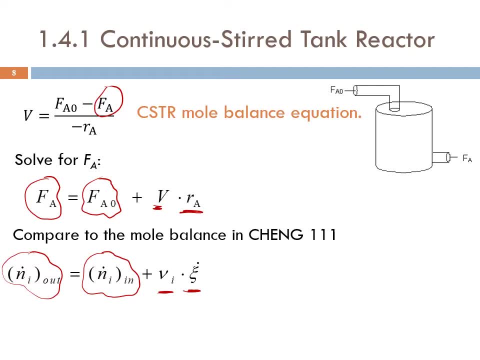 it's a flow system, so it's dot, not meaning it's a rate zeta, right, which zeta was the extent of reaction? extent of reaction for that specific reaction? okay, let's compare these equations. okay, let's compare these equations. okay, let's compare these equations. okay, let's compare these. 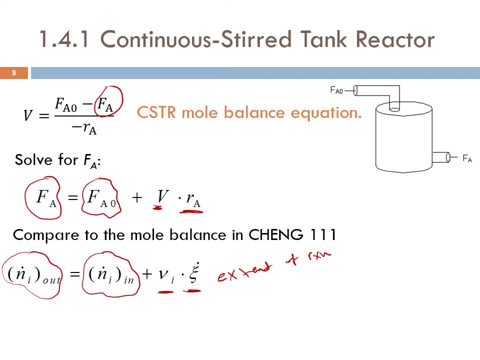 them. apparently they are the same right, because you have: output equals input plus plus the change right, plus the change plus the production or plus the generation term. okay, so they are the same: output equals input plus generation for a steady state system, for a steady state reactor. so let's see now, what can we do now? 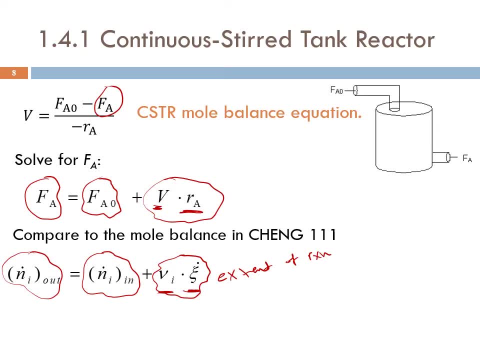 that we are grown up now in the third year, that we could not do in year number one, the first year, using this equation. okay, again, what can we find? what can we calculate now that we could not really calculate then in the first year? well, obviously, if you compare these two equations, you can see that 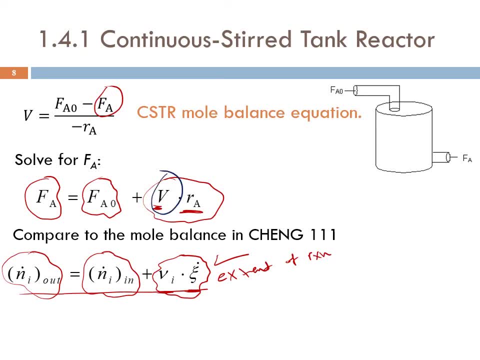 you can have v here, volume, right the volume. here you can calculate the volume. so, using the design equation, which is basically coming from the mole balance, i'm here able. i'm able to calculate the volume. how am i able to calculate volume? i'm unable to calculate volume through the knowledge. 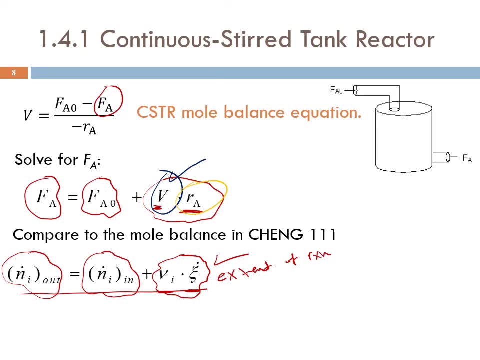 of the rate of reaction. i know the rate of reaction. therefore i'm able to calculate the volume to design the reactor. however, in triple one, in triple one, i did not really bother about the rate of reaction. i only have this, you know, collective, like overall number, which is the extent of reaction, and therefore i cannot really find the 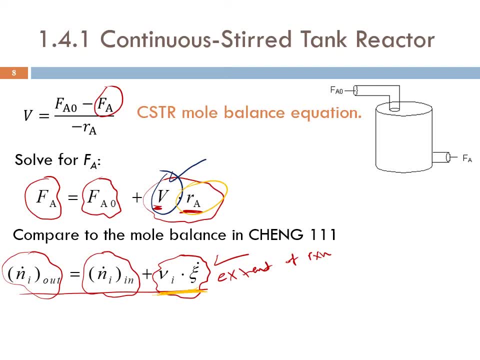 required volume to achieve a given conversion right and nu, which is the circumference number, simply something theoretical, right from the reaction. okay, so now that you're grown up, in the third year you are able to do more things with your knowledge, which is design. you are able to design here: design a reactor in order to design. 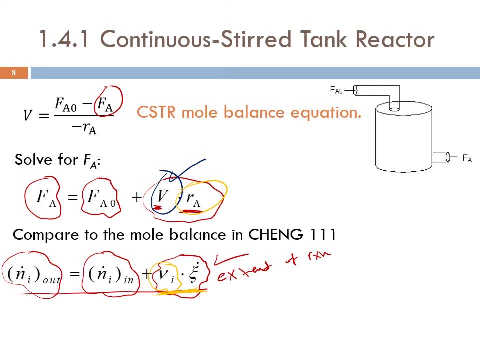 you need to know rate, correct, and the volume is proportional to the rate. because if the rate of reaction was large, if the rate of reaction was large, right, the required volume will be small. correct, because the reaction is happening fast, so you don't need large volume. and, of course, 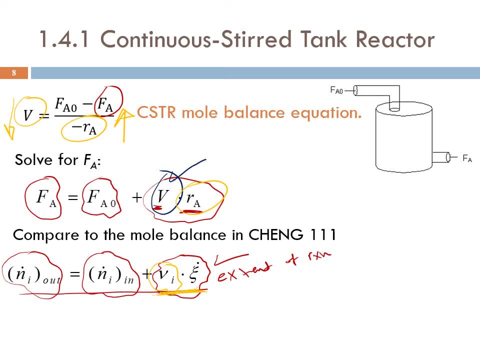 if you don't have large volume, that means the residence time. the molecules stay in the reactor for a shorter time, and that is fine because the reaction is very fast. i don't need the molecules to stay very long, okay, so remember the importance of the rate that it enables you to design, just like. 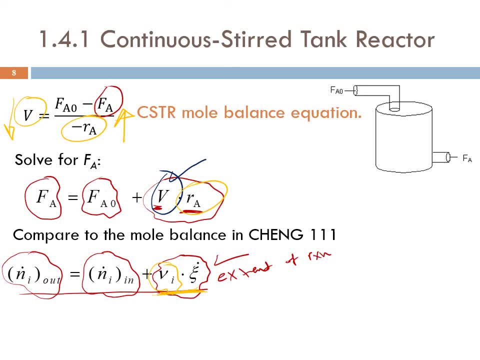 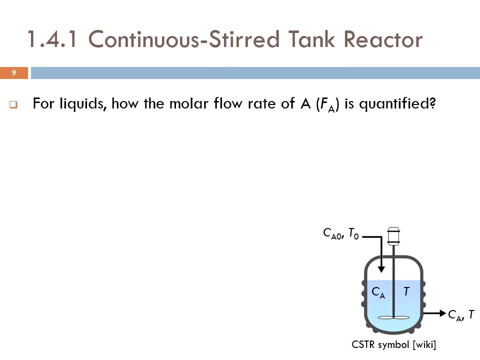 the importance of that rate of reaction. so the heat transfer enables you to calculate, to design the heat exchanger. but in the design of heat exchanger i'm not calculating the volume, i'm calculating the area, the heat transfer area. so that's the similarity. let's finalize for liquids how the molar flow rate of a which is, if a right, that's appear, this appears. 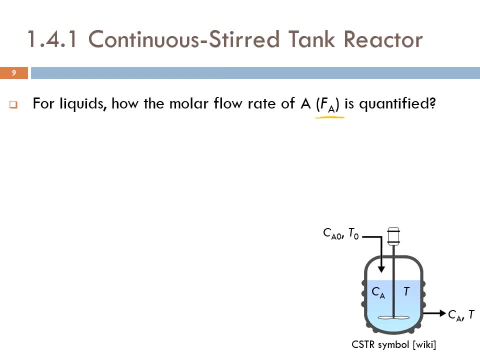 in the design equation quantified. okay, do we? this is the molar flow rate. do we use the- you know more- molar flow rate meter? do we do this or usually we do something else? if a can be calculated or quantified from the concentration ca and the volumetric flow rate, the volumetric flow rate which we refer to, 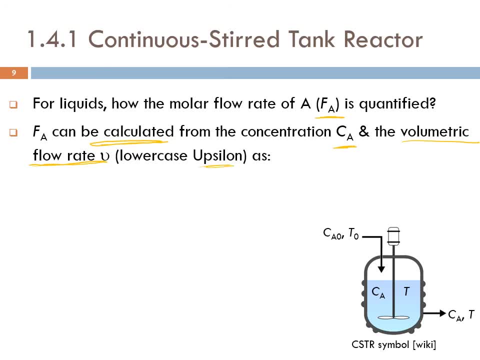 in this textbook as epsilon. epsilon, and it's the lower case. it's an epsilon with a billy, okay, and how is it quantified? by this equation? of course, whenever you forget it, okay, you can really check the units. let's check the units together. okay, so ca? ca could be mole per liter. and what is epsilon? which is the volumetric flow rate it's. 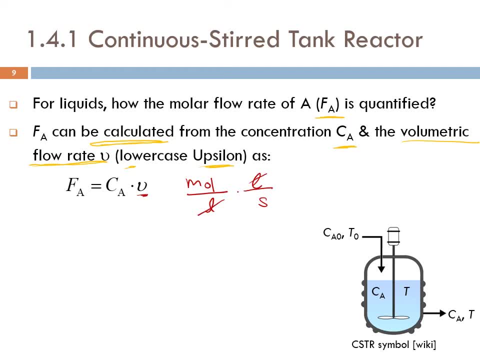 liter per second. so if you cancel the liter you get mole per second. mole per second, which is the molar flow rate. so if you want to measure the molar flow rate here, you can calculate. sorry, if you want to calculate the molar flow rate here what you can. 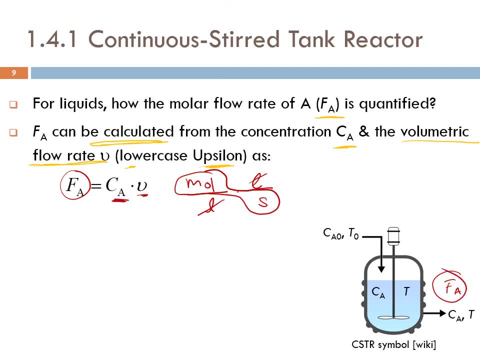 do is you can measure the concentration here and the stream multiplied by the measured volumetric flow rate. so you can easily measure concentration. you take a sample, take it to the lab and analyze it. you get the concentration, whether you're going to use the volumetric flow rate or you're going to. 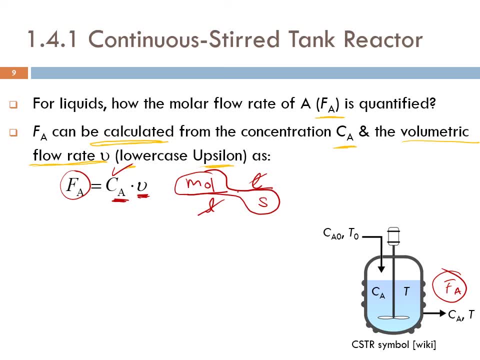 use a spectrophotometer, you're going to use the gas chromatography, you're going to use the titration, whatever you're going to use to calculate the concentration of a. and then you calc, you also measure. you measure the volumetric flow rate. okay, you measure the volumetric flow rate.